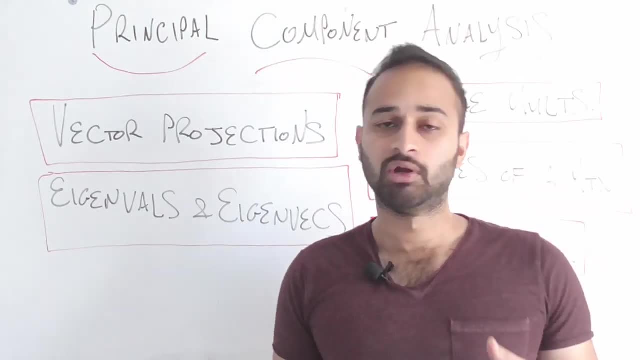 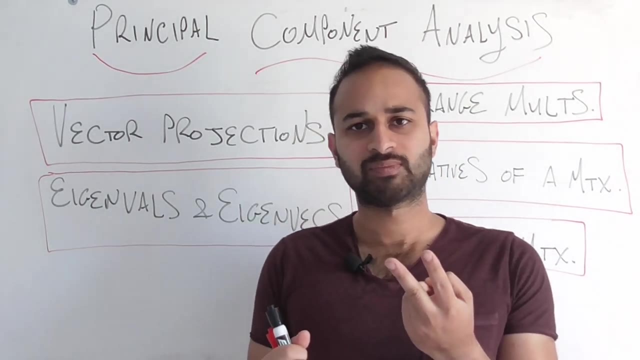 We're going to be taking several derivatives of matrix operations in this video, so it helps to be familiar with that. The last one will be covariance matrix. There are actually two videos on the covariance matrix. one is on the introductory to what a covariance matrix is. 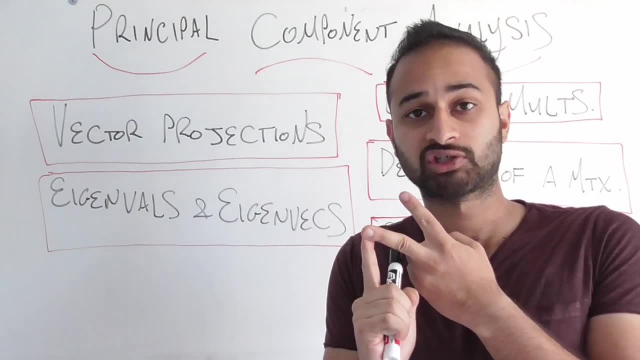 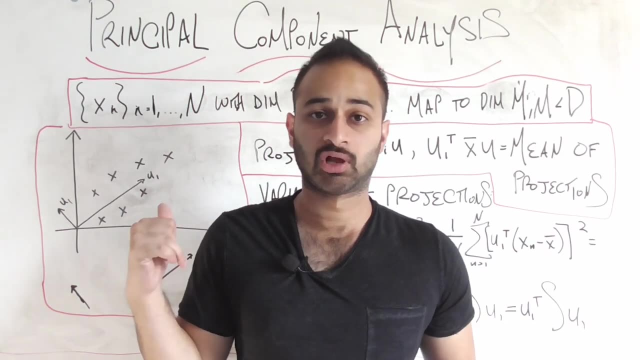 the other is the enclosed form of a covariance matrix. Okay, now that we've talked about the different math videos that you want to watch to have a good foundation for what's coming up in this principal component analysis mathy video, let's go ahead and get into it. 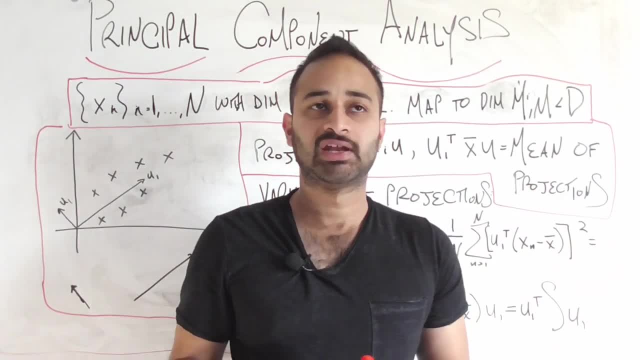 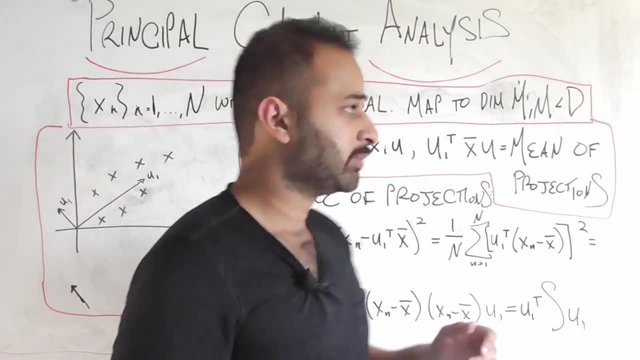 So it looks like there's a lot of kind of ugly math behind me, but I promise that if you have watched those previous videos and are kind of comfortable with the results, then this will go a lot smoother. And also I'll be going through it slowly. I'll be taking it step by step, so don't even worry, okay. 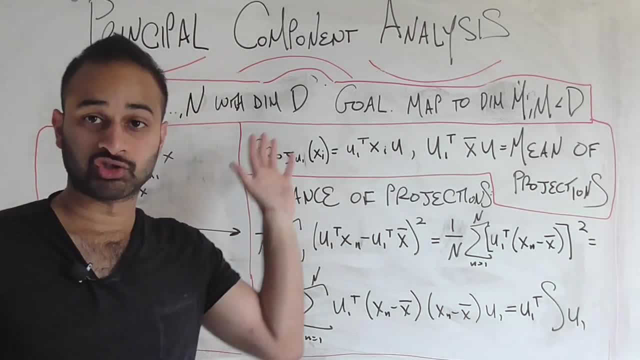 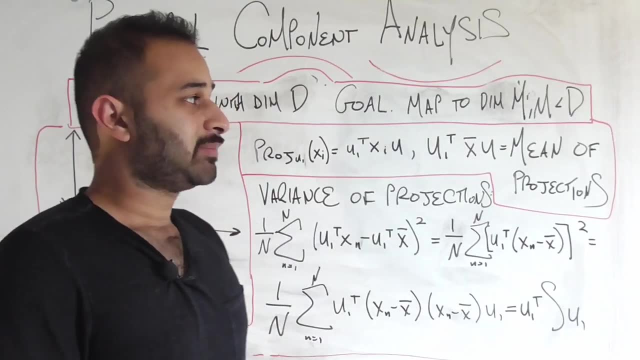 So I put stuff in these little red boxes so that we can keep the logical progression a little bit easier, because there's a lot more moving parts in this video. So the first one is just: what's the setup? So the setup is that we have n different vectors- x1, x2, all the way to x, big N- and they have together dimensionality D. 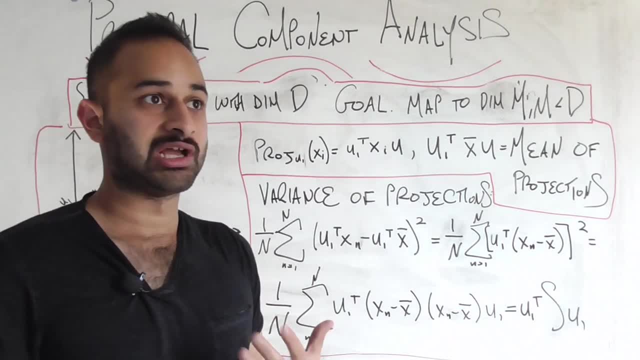 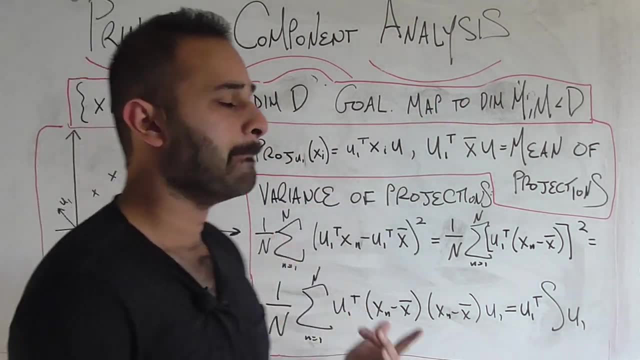 Our goal, of course, in principal component analysis is dimensionality reduction. So we want to map this space which has dimensionality D onto a space which has dimensionality M, where M, of course, has to be less than That's the point of dimensionality reduction. 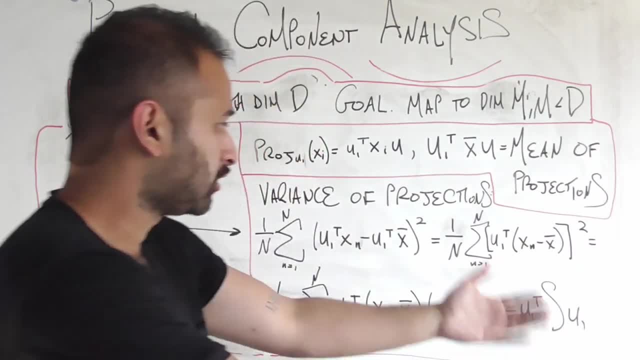 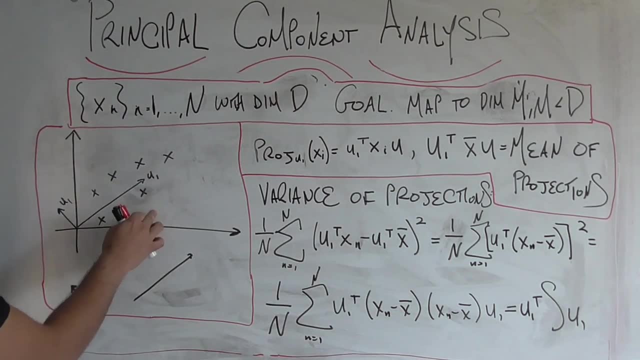 How are we going to do that? Seems like a daunting task, but let's take a whole step back and let's look at a simpler picture. Let's say that we have again these points here, So this you probably saw from our projections video: the same setup. 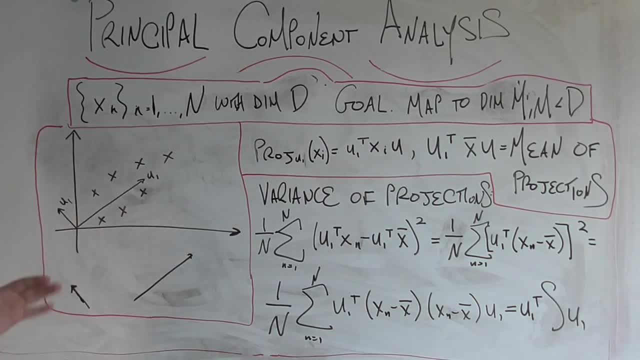 So we have all these different points here and we want to figure out if we're just going to map it onto a one-dimensional space, so vector u1 somewhere in this space, then which u1 should we choose? Here's just two candidates to help us kind of get started thinking about. 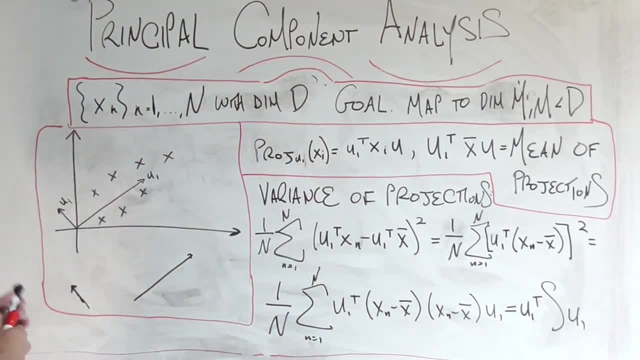 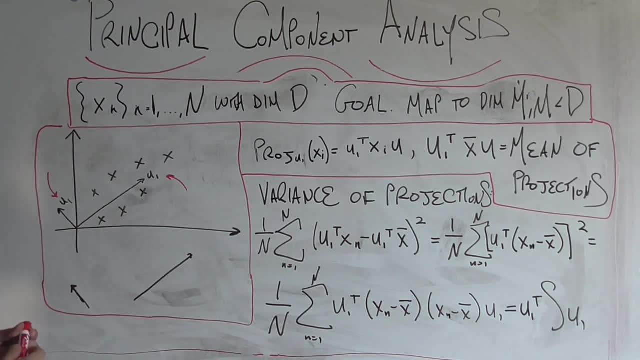 what's a good criteria for picking such a u1.. Let's say, one candidate for u1 is this guy. a different candidate for u1 is this guy. Now let's say we go ahead and project our data onto this guy, this candidate for u1, then what's it going to look like? 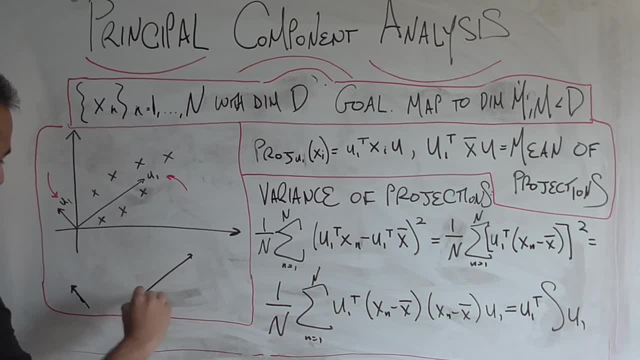 So here's that candidate for u1.. It looks like one of the data points will be here, one will be here, one here. I won't draw all of them exactly, but they'll be kind of evenly spread out among this u1 vector. 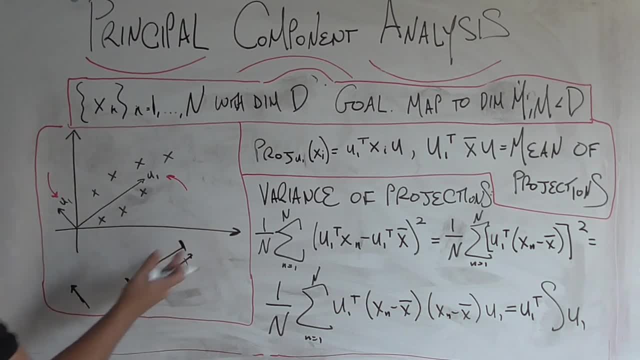 and there will be a lot of variation preserved. So kind of this. the length of this vector it's not exactly, but it's kind of a proxy for how much variation is preserved from the original data set. Now what if we choose to instead project it on this different vector u1 down here? 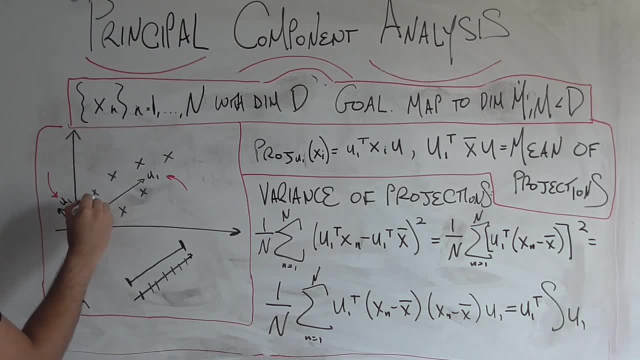 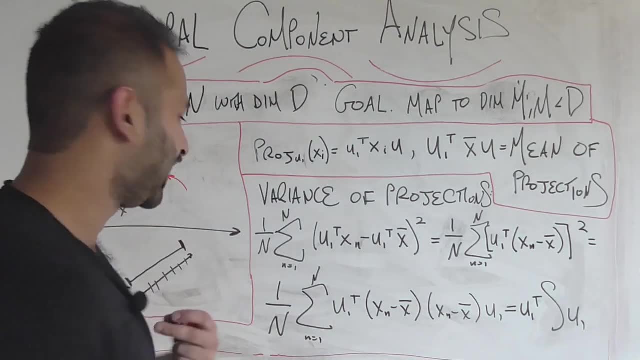 Then there's a different story, right? Because, for example, if we take this vector and project it down here, there's not a ton of variation preserved, And that's kind of the criteria for how we're going to select the best u1 to project on if we're just trying to project onto a one-dimensional space. 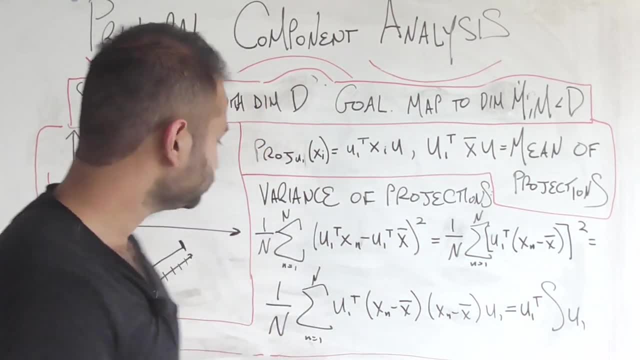 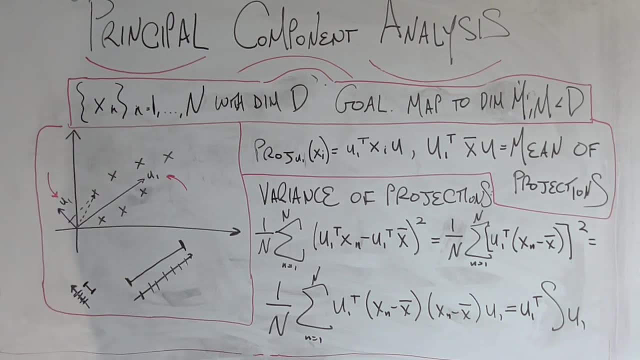 So that's if m is equal to 1.. Right, So we see that the criteria is that we want to maximize the variance of the projections onto this one-dimensional space. What that kind of means is a more human context, is that we have this d-dimensional space. 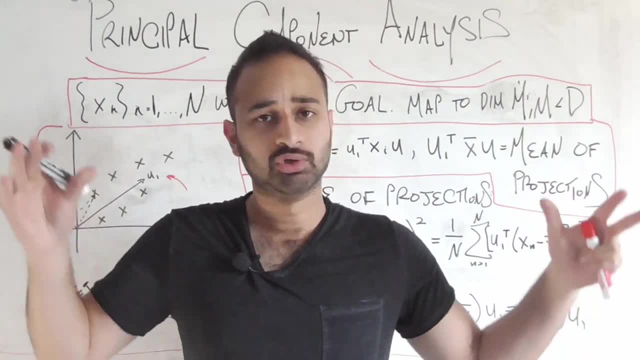 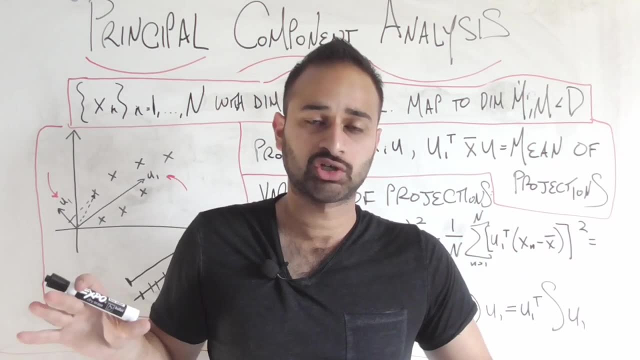 it contains all this information, all this data. We want to reduce its dimensionality, but we want to do it in a clever way. We want to do it onto a space so that we preserve as much of the original variation as we can, while reducing the number of dimensions. So there's dumb ways to do it, Like if we use this u1,, we want to reduce the number of dimensions. So there's dumb ways to do it, Like if we use this u1,, we want to reduce the number of dimensions. 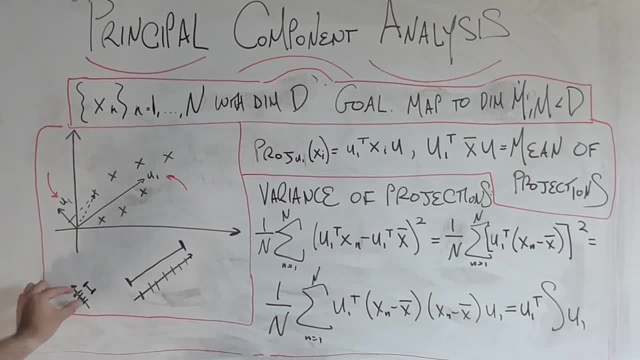 So that we preserve as much of the original variation as we can while reducing the number of dimensions, So that we preserve as much of the original variation as we can while reducing the number of dimensions. And if we use this u1, we would be losing a ton of information because everything kind of just compresses into this little space. 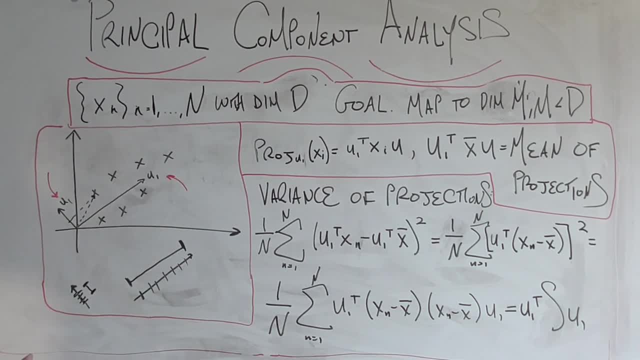 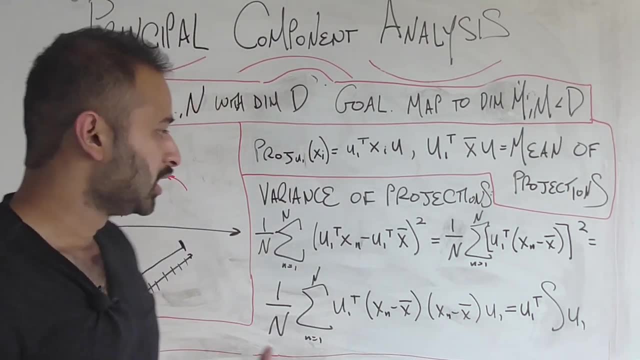 But there's smarter ways to do it. We can use this vector so that we still get a one-dimensional space in the end, but we're preserving this much variation instead, which is a lot more variation. So the question is: how do we figure out mathematically what's this best? u1 to project on. 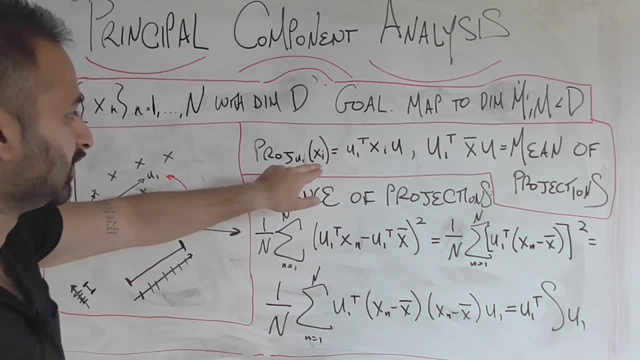 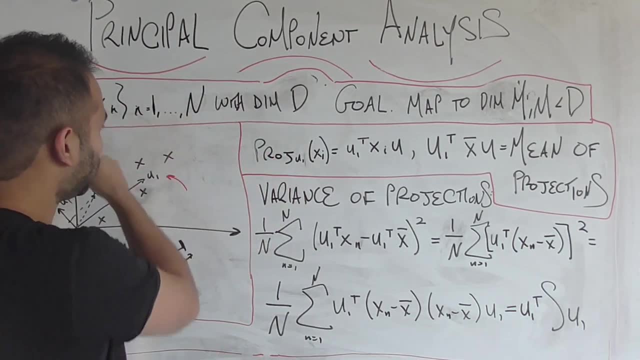 Well, let's first write out the formula for the projection for any given data, point xi. This is coming from the projections video, So remember the projection of of xi. this is a vector in our set onto a potential u1 vector is going to be u1. 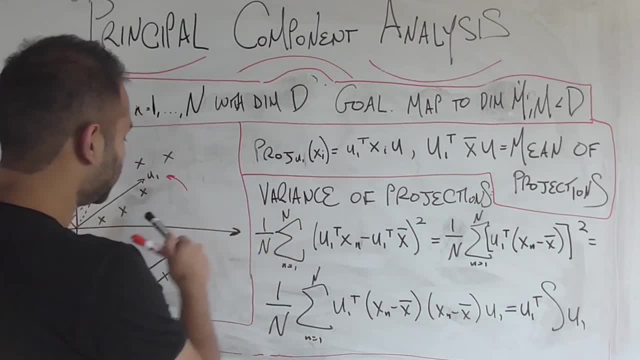 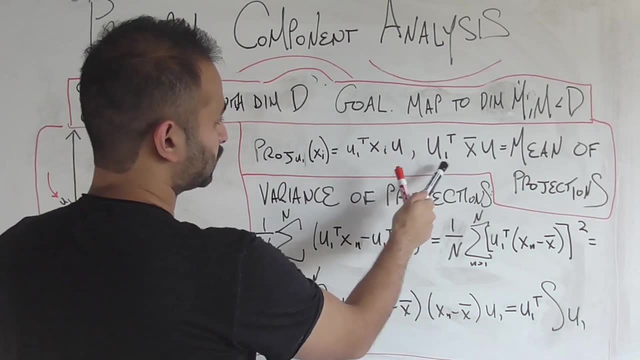 transpose xi: u. okay. u being a unit vector: okay. So then also the mean of all of the projections, so of all of our data, is going to be u1. transpose x bar, x bar being the mean of all of our x's: u. So this is, this makes sense because it's. 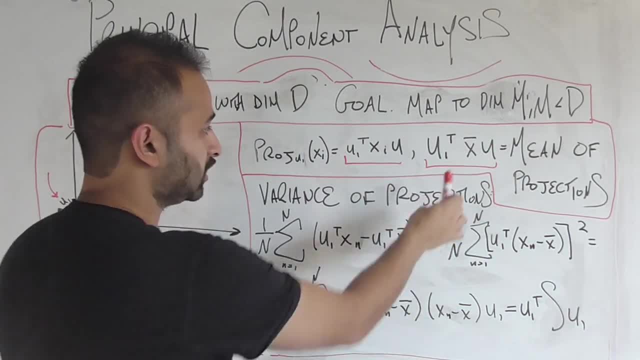 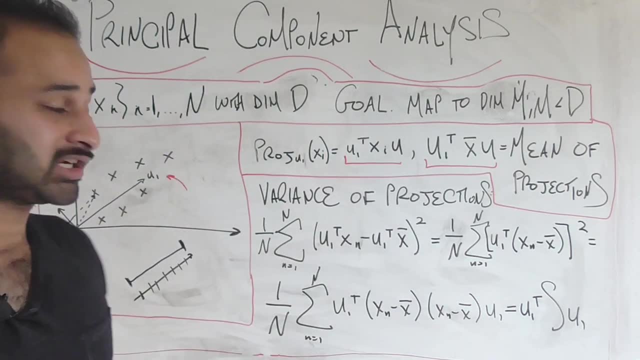 just an analog to this and since the mean is a linear operation, it behaves in the exact same way here. so that's the mean of the projections. Now, again going back to our objective, our objective is to maximize the variance of the projected data. Variance is basically just taken by. you know their classic. 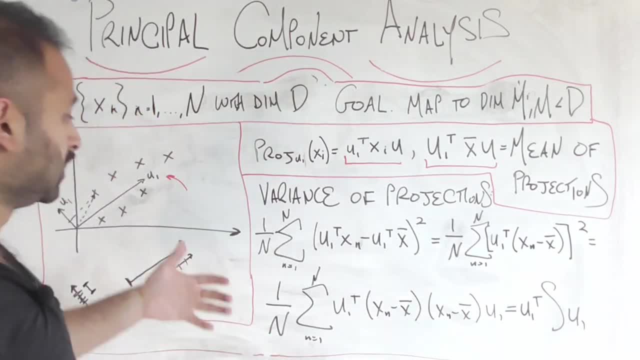 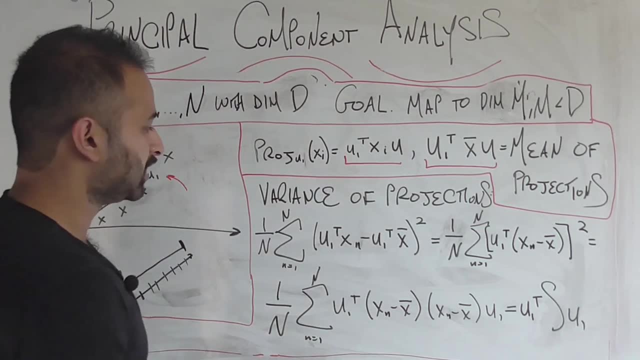 variance formula from stats 101 or your initial stats class, is 1 over the number of variables. you sum over all of the different variables, all the different vectors we have here, and we basically subtract the length of each vector. so this is the length of the vector right, Because this is the projected form of 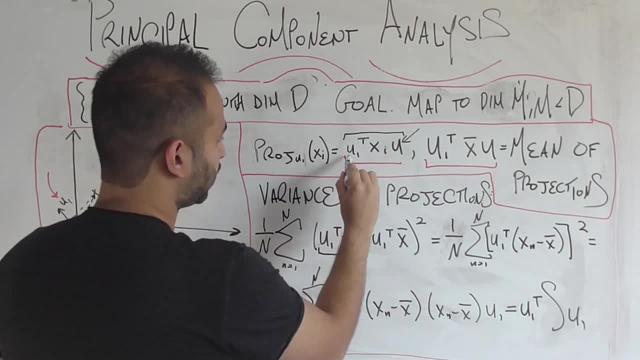 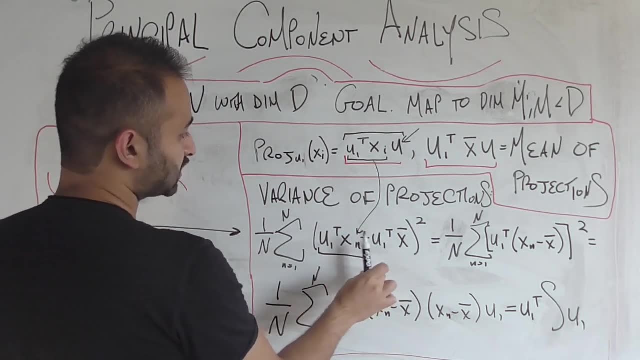 the vector and this is the length of the vector right, Because this is the projected form of the vector and since u is a unit vector, its magnitude is given by just this piece right here, which is the same thing written here. So the length of the projected vector minus. 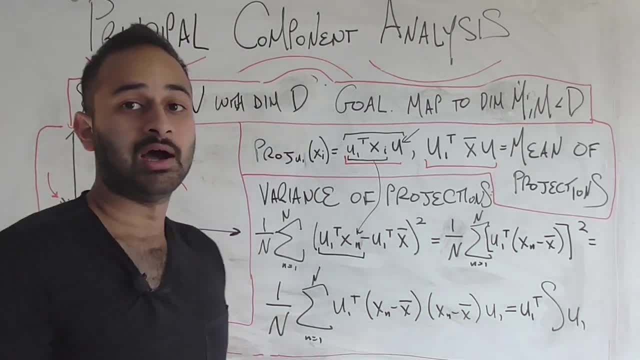 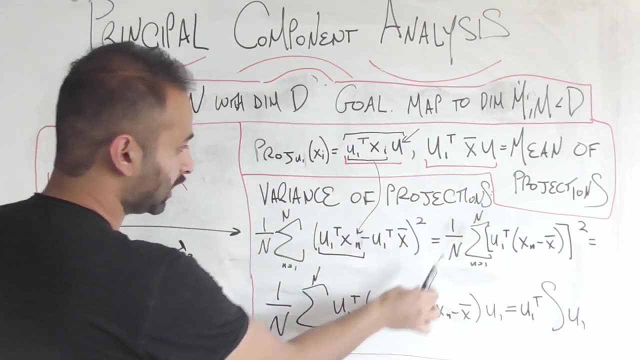 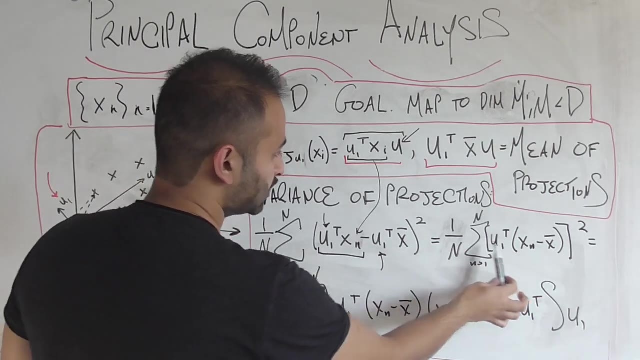 the mean of all projected vectors. remember, variance is found by taking the quantity minus the mean of all the quantities and you take the difference, square it. That's exactly what we're doing here Now. we're gonna factor out this: u1 transpose, u1 transpose. that's going to come out to the front and we 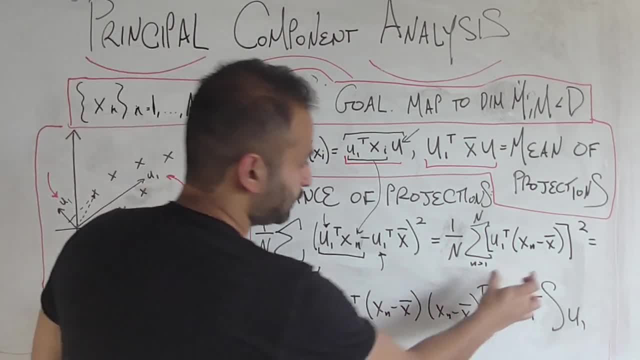 still have the same formula squared. Okay, now the next thing I want to do is expand this guy a little bit, so I'm gonna. this is squared right. So the first one I'm gonna leave exactly as it was. u1. 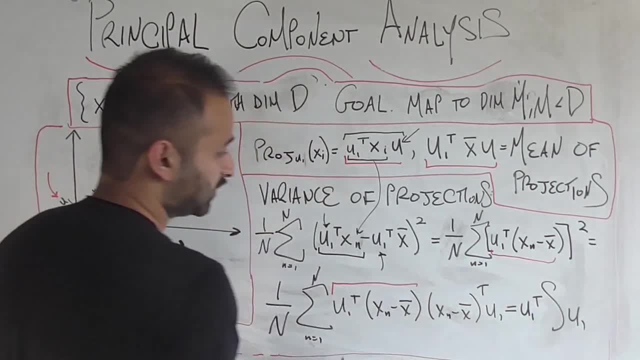 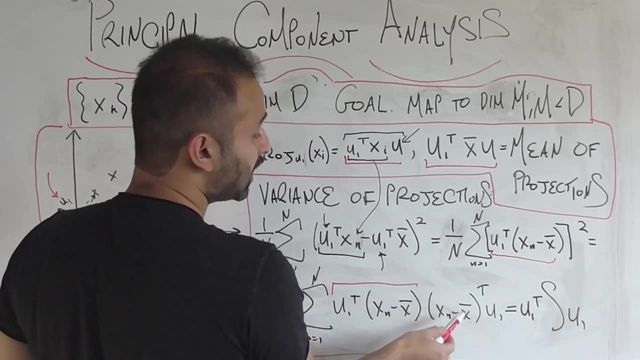 transpose: xn minus x bar. that's the first thing. The second one: I'm gonna rewrite it in the opposite way. So I'm gonna put the transpose on this guy- the xn minus x bar, first, and then write u1.. Quick break, why am I allowed to do that? 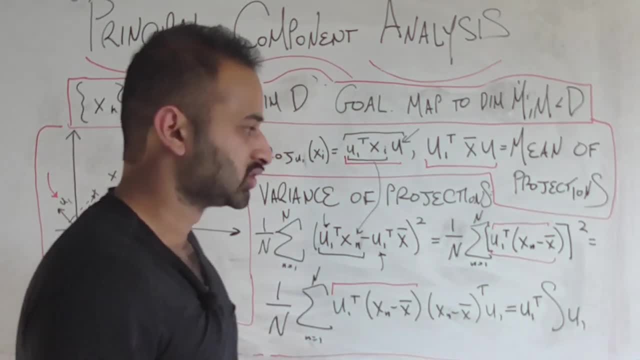 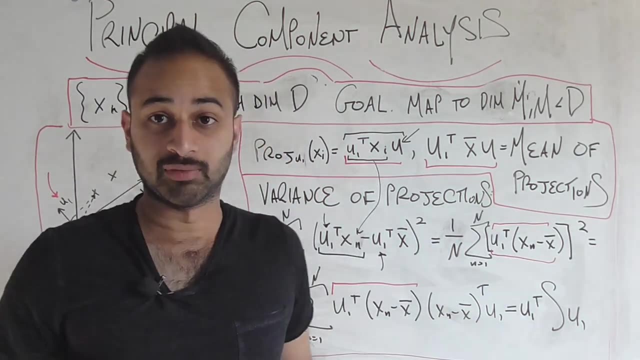 Well, because in the end, the thing inside here is just a number. so it doesn't matter in which order I take the transpose, If I put the transpose on the first vector or if I put on the second vector and write that one, it doesn't really matter. So that's why I'm allowed to do. 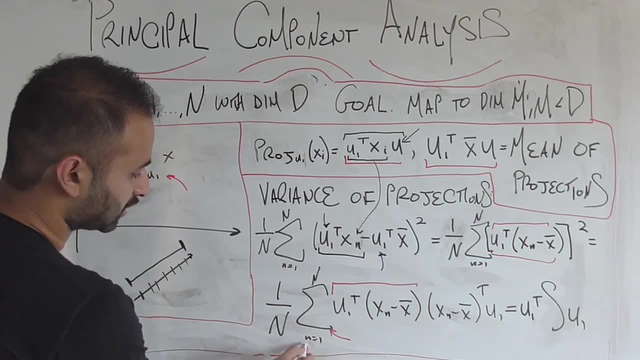 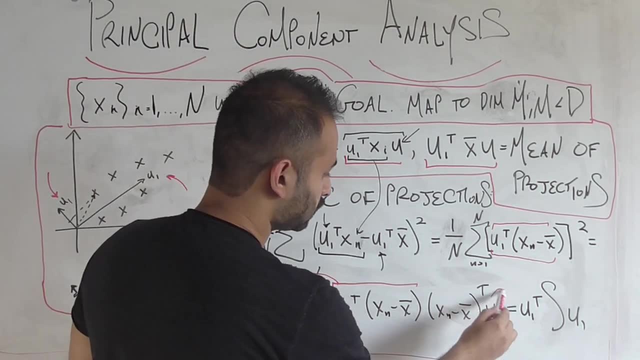 this. Now, since this sum only cares about stuff with the little n in it and u1 doesn't have any little n in it, I'm safe to kind of factor the u1 transpose out and out. And now what's left? So let me actually just write the u1 transpose on. 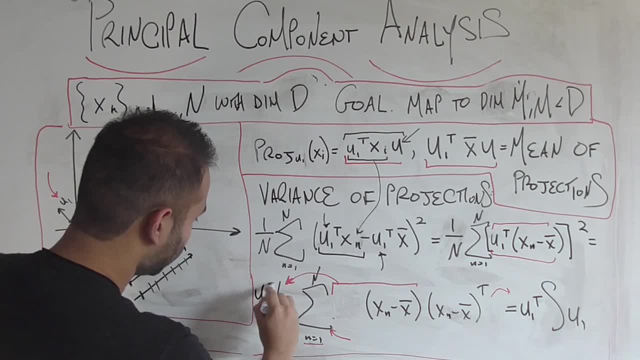 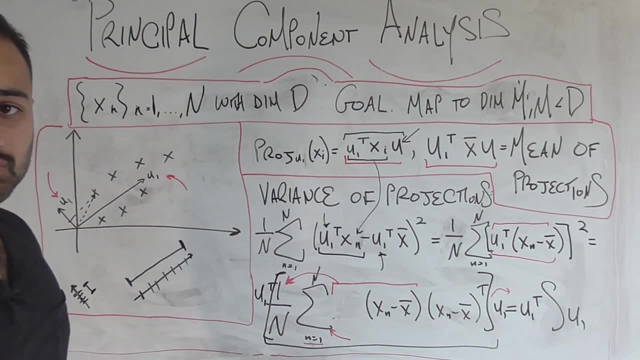 the outside. I'm gonna write it on the very outside, including this 1 over n here. What is this guy, this beast right here? So this beast right here. this 1 over big N sum from n equals 1 to big N of xn minus x. 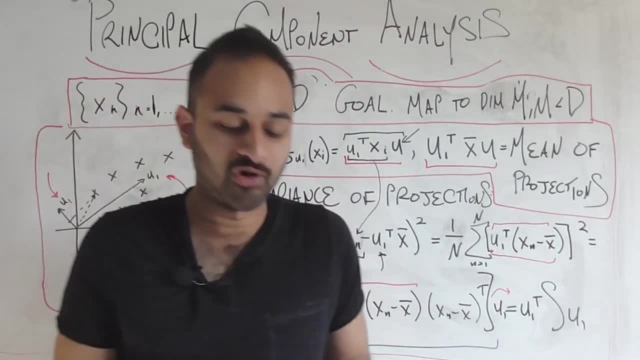 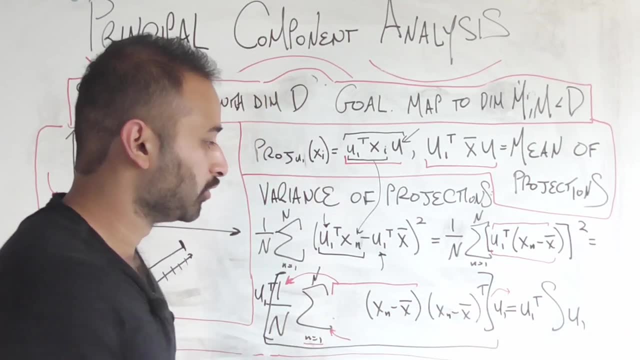 bar xn minus x bar. transpose that beast. if you go back to our video on the closed form of the covariance matrix, is the closed form of the covariance matrix, which is s. So that's u1. transpose s- u1.. Let's take a break, okay. 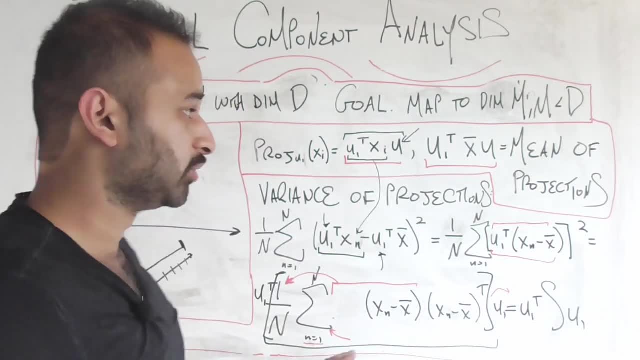 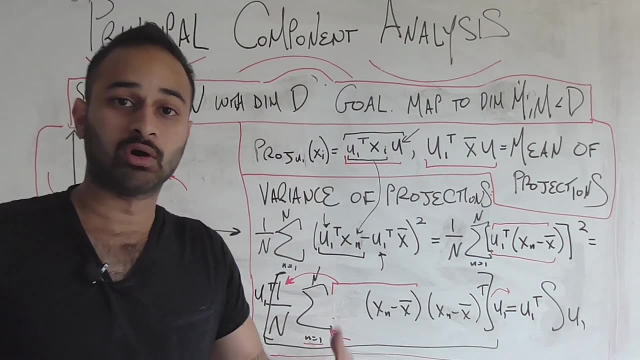 So we just did a bunch of math. we used a bunch of ideas already. we've already used the idea of the covariance matrix, the projection, okay, So make sure you're comfortable with all this. If you need to rewind, go ahead and rewind and become. 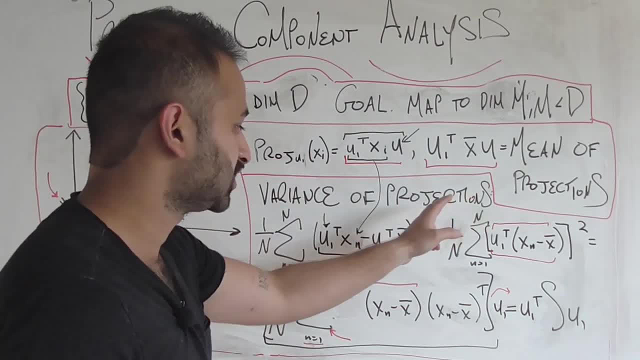 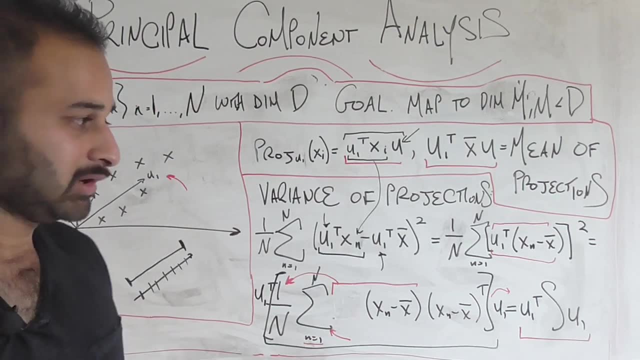 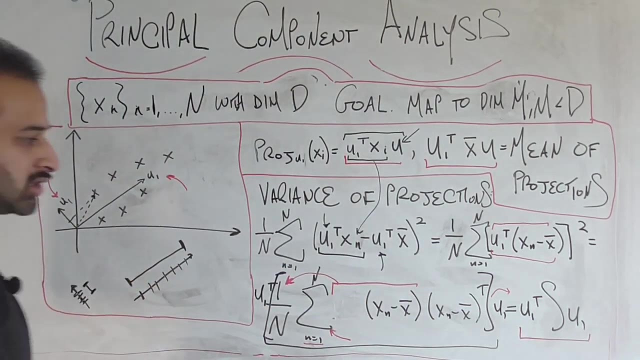 comfortable with the idea that the variance of the projections is given by this awesome closed form u1. transpose s the covariance matrix u1.. Okay, so now I'm going to erase the board and then we're going to try to maximize the variance of the projections. remember, that's our goal. subject to the. 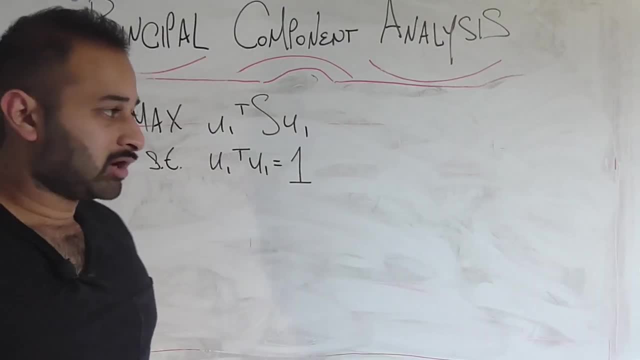 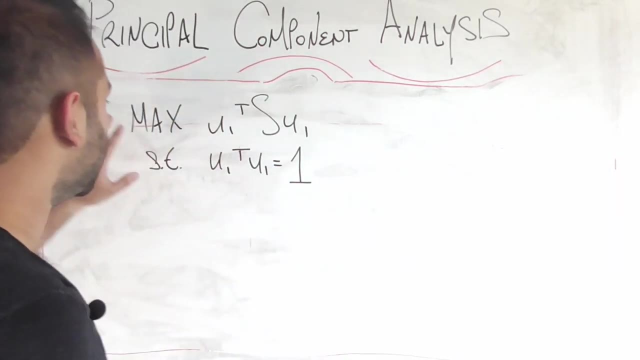 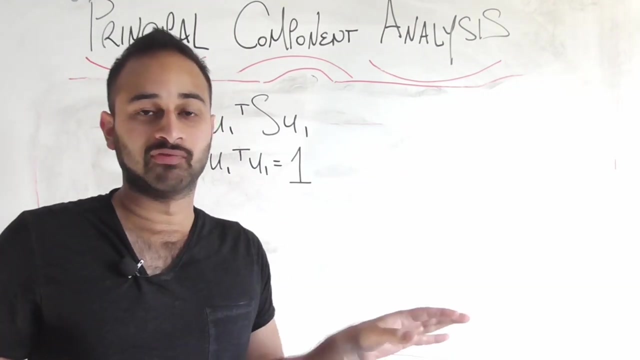 constraint, that u1 is a unit vector. Okay, and we're back. The good news is that we're done with the hard part of this video, The math we did before just setting up this. this maximization equation is the hard part. Why? Because the next stuff we're going to do is an exact repeat of 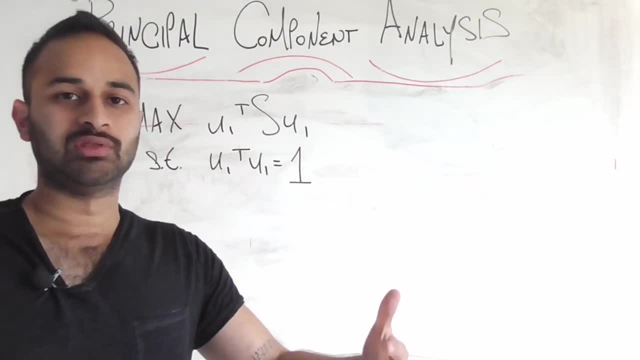 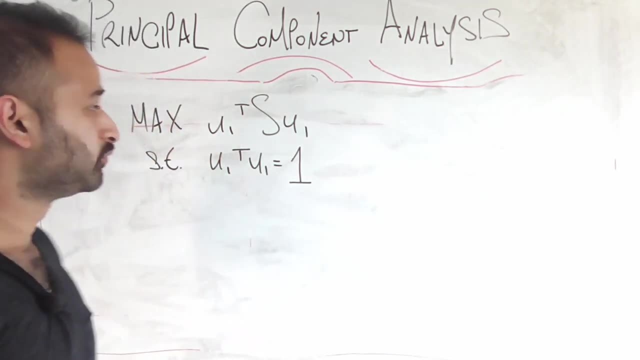 the problem we did in the Lagrange multiplier video. That's the reason I wanted to do that problem back in the Lagrange multiplier video, so that now it's already been done. But you know what We're here, let's do it again. So we want. 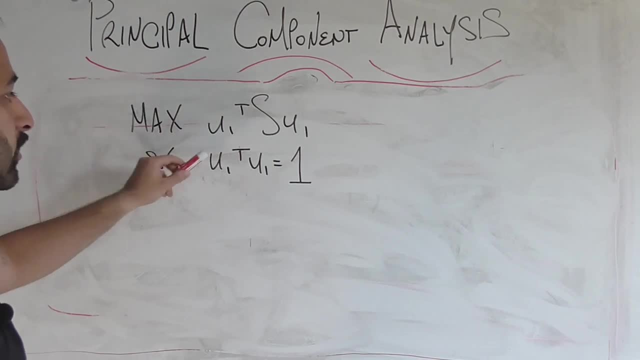 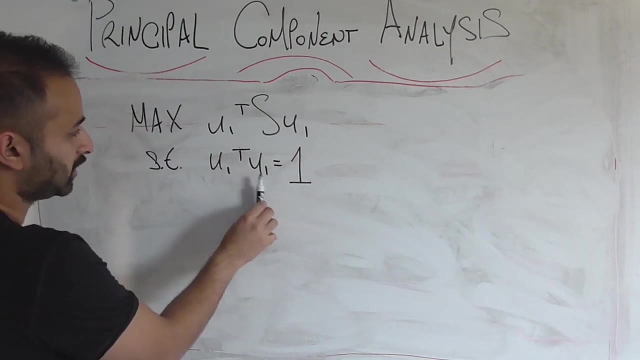 to maximize the variance of the projections which, as we just found, is u1, transpose s the covariance matrix u1, subject to the constraint matrix. okay, So we can just say here that u1 transpose u1 is equal to 1, which. 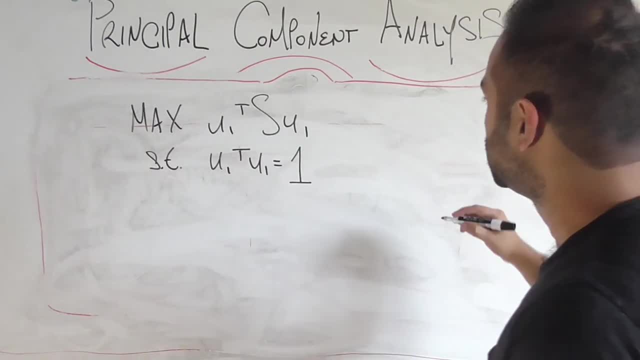 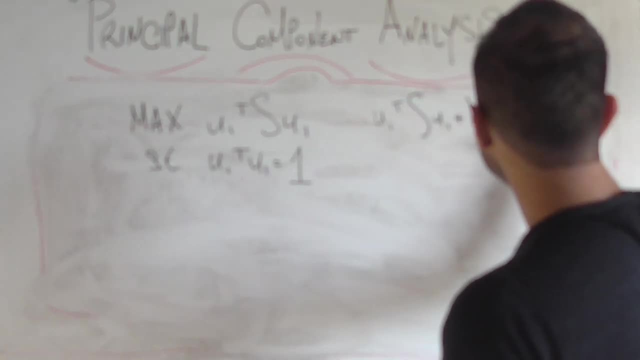 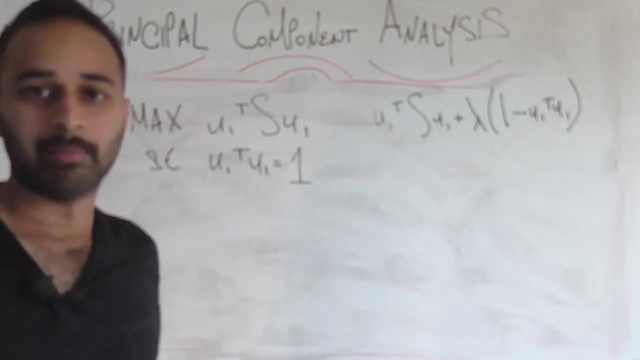 just means that u1 is a unit vector. okay, So, using the power of Lagrange multipliers, we have a new objective function which looks like: u1 transpose s, u1 plus lambda. 1 minus u1 transpose u1.. Okay, so that is the new objective. 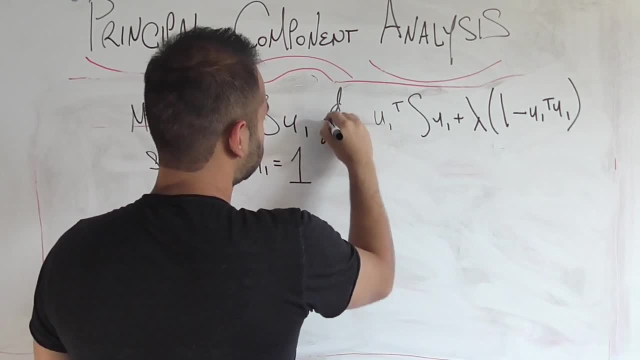 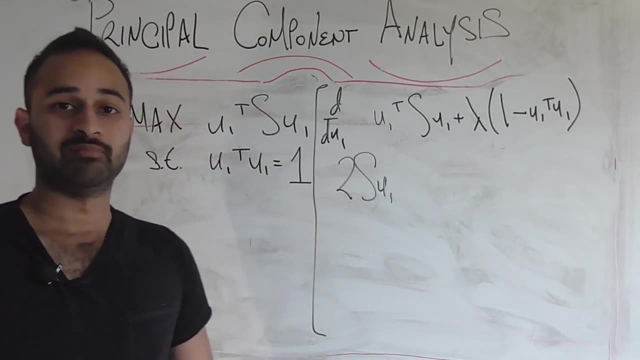 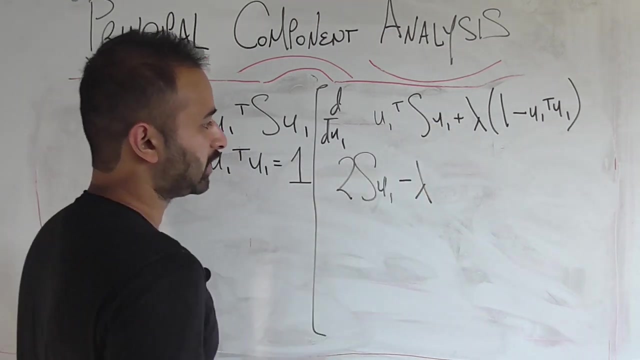 function that we want to maximize. So if we take d du1 of that guy, we're going to get 2su1.. This is coming from the derivative of matrix operations, video Plus, I guess it's going to be a minus. actually lambda, which is just the Lagrange multiplier itself. times 2u1 equals 0.. 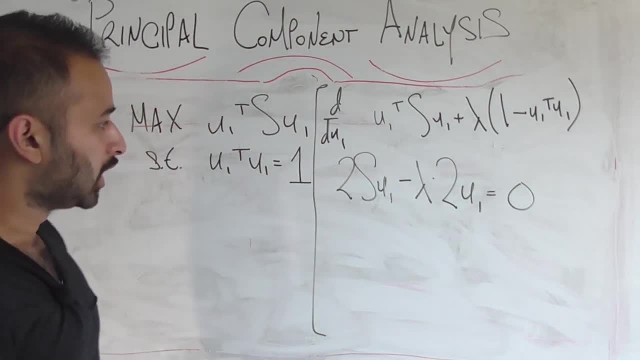 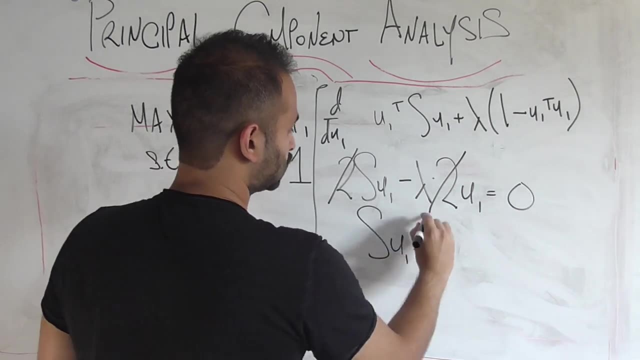 We're going to set it equal to 0 because it's a maximization, minimization problem. Now it's pretty simple. We're going to cancel out the 2s. We're going to move this guy to that side. We're going to get: su1 is equal to lambda u1.. 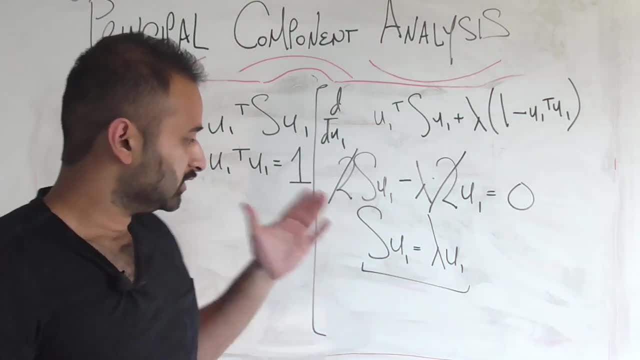 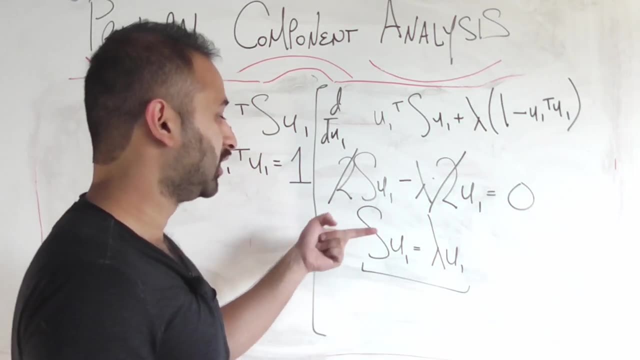 What does that mean? Again, like in the Lagrange multiplier video, this means that u1, whatever direction we choose to project on- is going to have to be an eigenvector of the covariance matrix S, because this is the definition of an eigenvector. 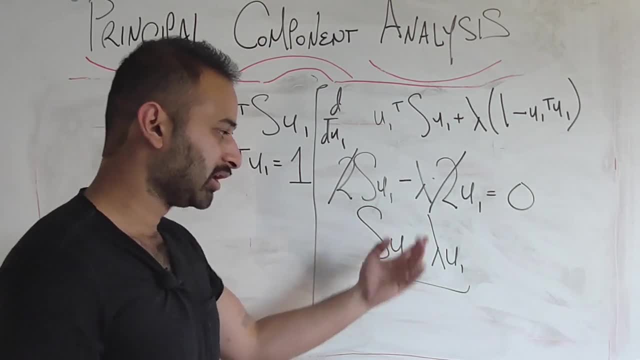 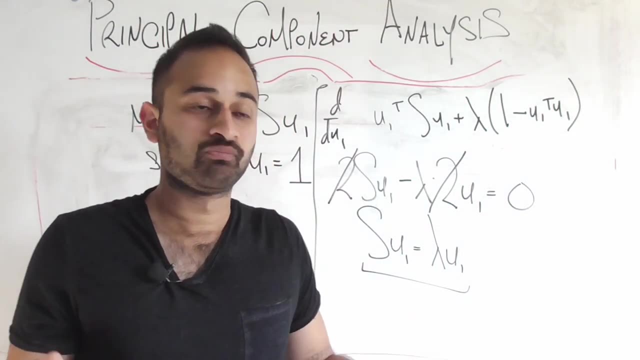 is that S times u1 is equal to some multiplier, lambda times u1.. But which eigenvector, which eigenvalue do we use? Because S could have many. To figure that out, let's hit each, both sides, by u1 transpose. 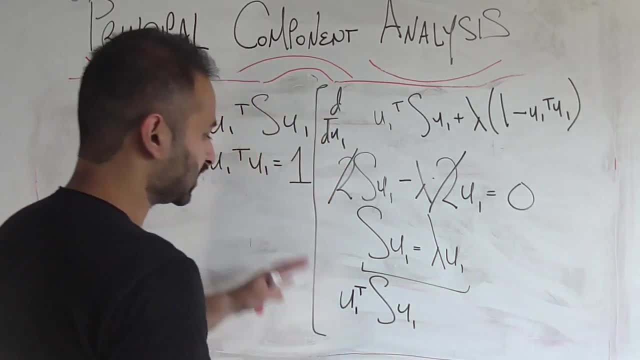 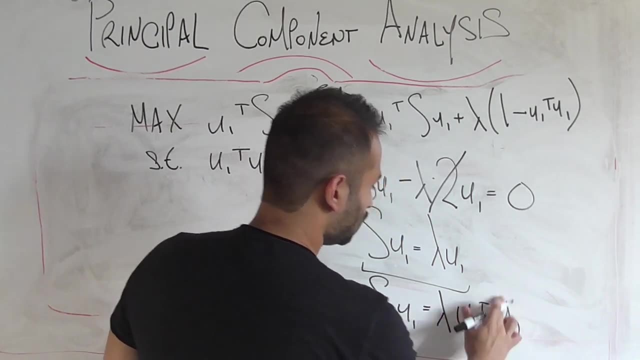 So we get u1 transpose su1.. I've just left multiplied by u1 transpose. I'll do the same thing here. Lambda being a constant can just come right out. Okay, so we have this formulation here. What is u1 transpose u1?? 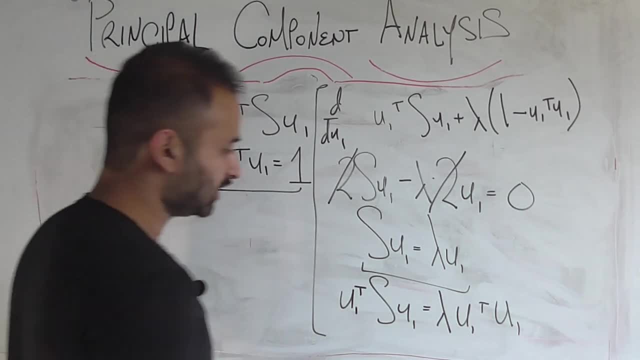 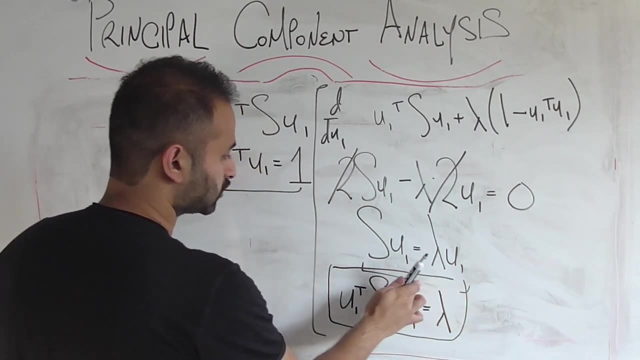 Of course that's equal to 1, from what we stated initially. So this guy just goes away And we get this result that u1 transpose su1.. u1 is equal to the Lagrange multiplier lambda. How does that help us figure out which eigenvector to use? 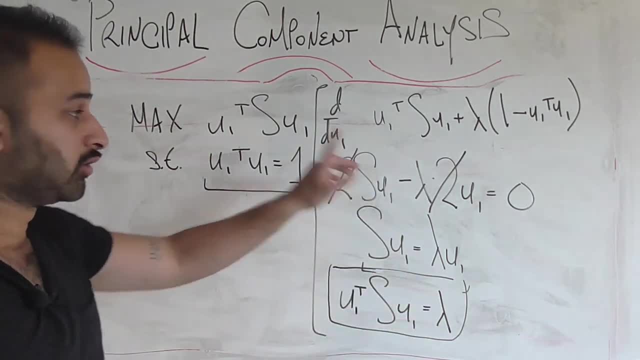 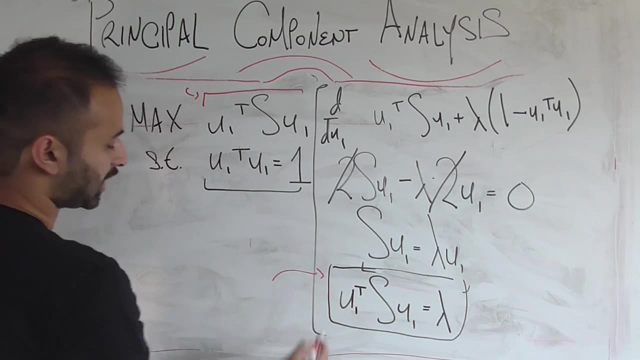 So, if you notice again, u1 transpose su1,. going back, here is the initial thing that we were trying to maximize in the first place. So this guy matches to this guy. So if we want to maximize the left side of this equation, we same thing as maximizing the right hand side of that equation. 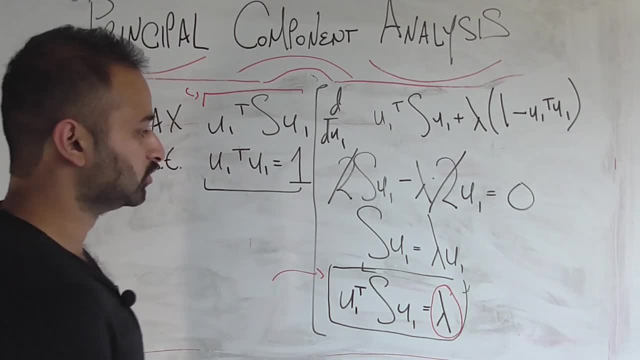 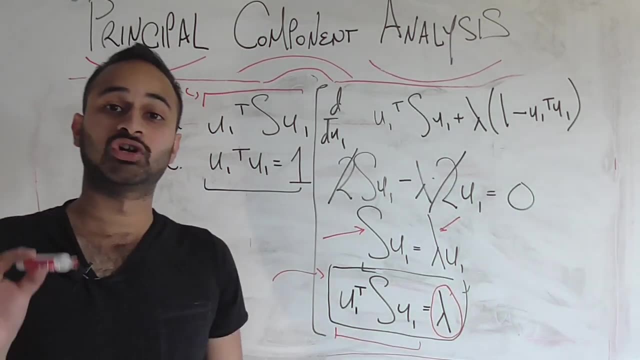 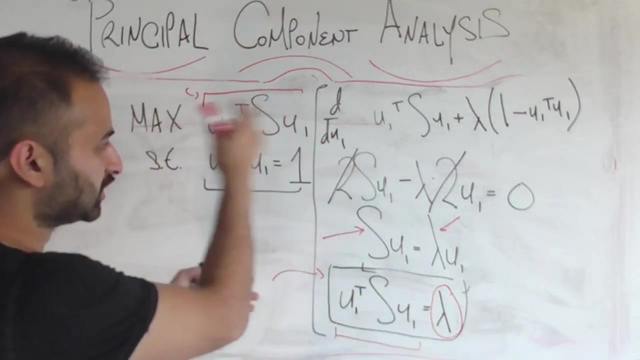 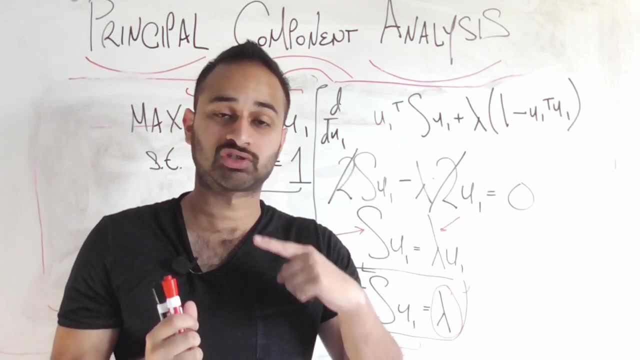 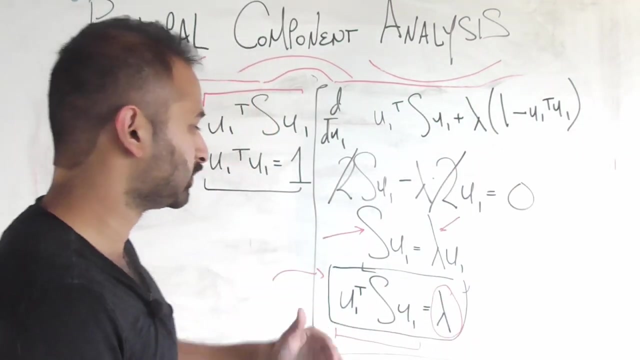 So we're going to pick the biggest eigenvalue of the covariance matrix S, because that's going to give us the biggest value for the variance of the projected data, which is exactly what we wanted to do. So I know that's a lot of tracing through these equations, but the result, the final result, is that if we first want to just pick which one dimensional space to project our d dimensional data on, what we're going to do is figure out all the different eigenvalues of the covariance matrix S. 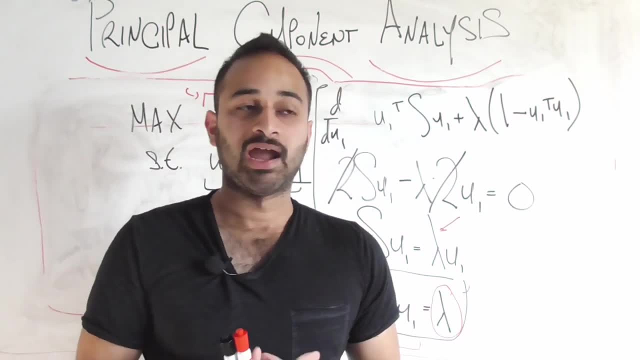 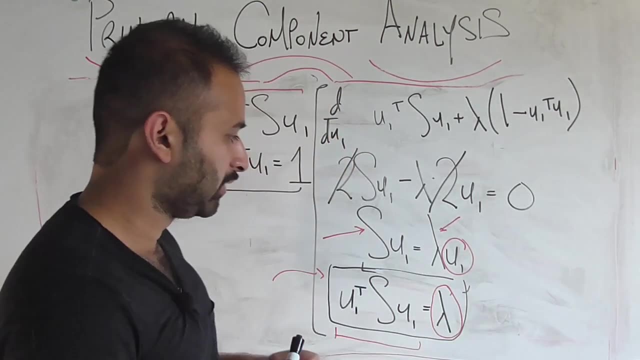 Pick the biggest one, right, The biggest lambda, And then figure out what is the eigenvector that matches up with that eigenvalue, And that's going to be u1.. Of course we want to make sure to normalize that eigenvector. 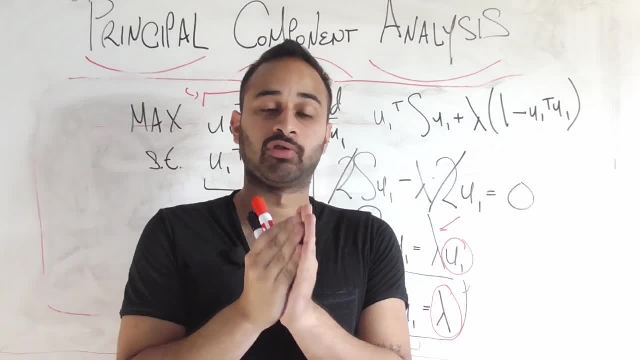 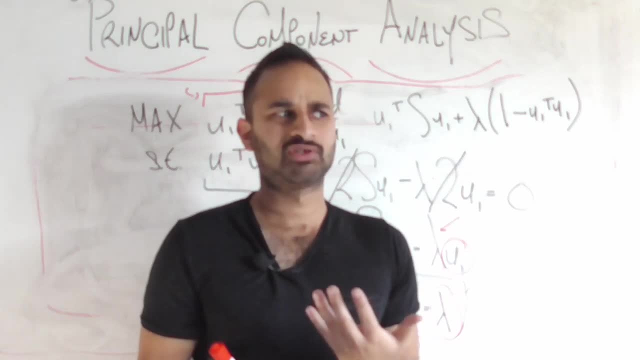 So it's a unit vector And that is the answer for the one dimensional space that we want to project on first, onto our data. Of course, your question is now: okay, that's projecting on a one dimensional space, but I probably want to project on a higher space, right? 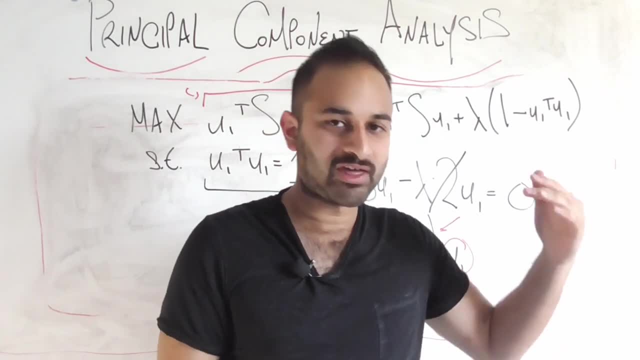 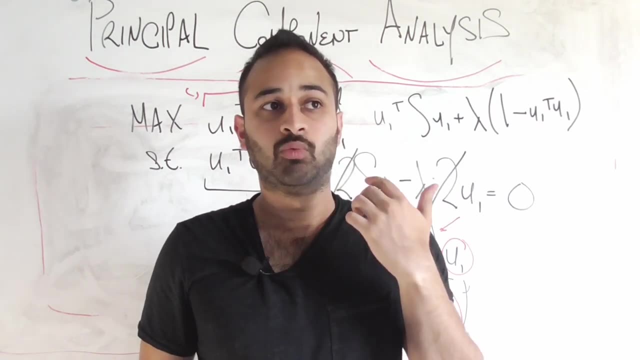 Maybe four or five, whatever dimensional space. Well, you can use mathematical induction on this one. We won't. We won't get into those details, but the result, the awesome result, is that, okay, let's say you want to figure out what are the best two dimensions to project my like 10 dimensional data on. 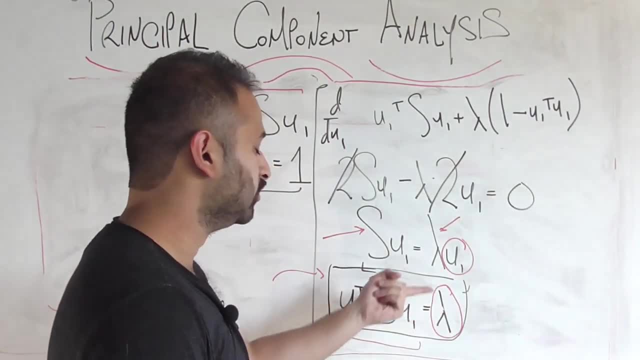 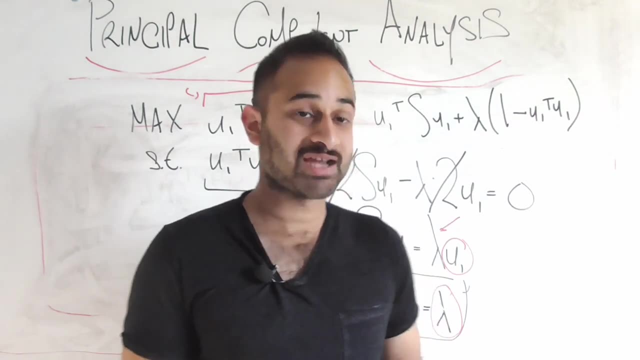 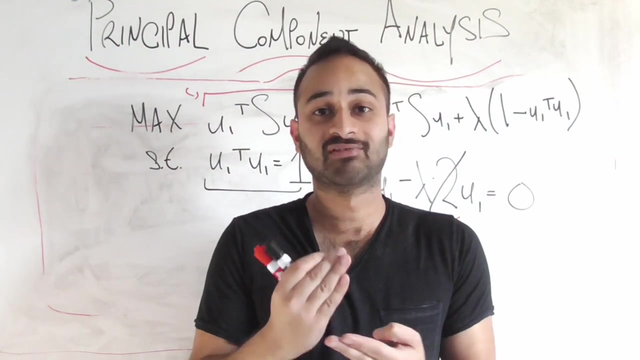 To get the first one, you figure out what's the top eigenvalue and you find out the corresponding unit eigenvector. for the second one, You figure out what is the second biggest eigenvalue, the biggest lambda after the initial lambda, and you use the second biggest, use the eigenvector corresponding to that second biggest eigenvalue. 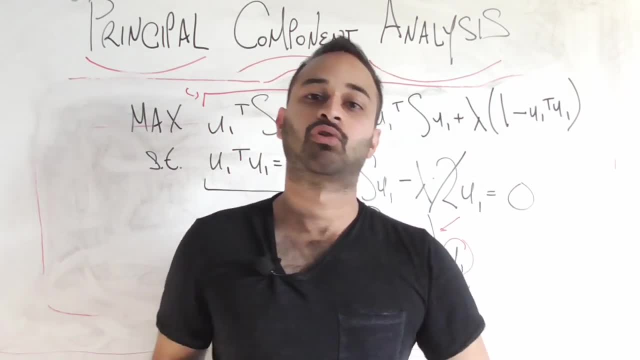 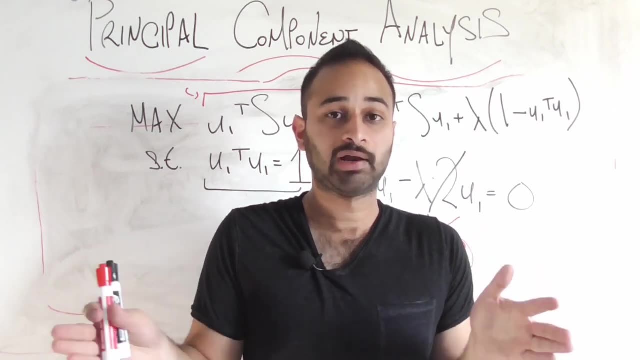 For the third one, use the third biggest eigenvalue and the eigenvector corresponding to it, And that's it. You just go down in line for however many different components you want, whatever dimensional space you want to end up in, And that's how you would arrive at them. 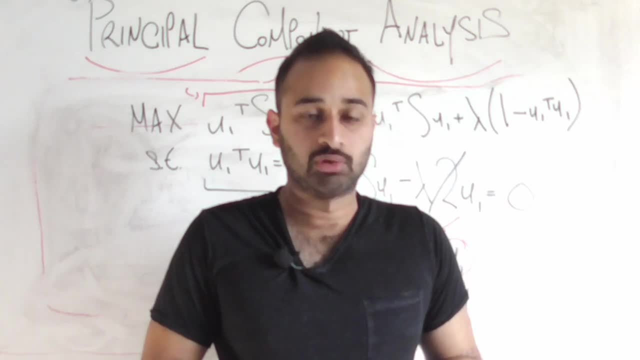 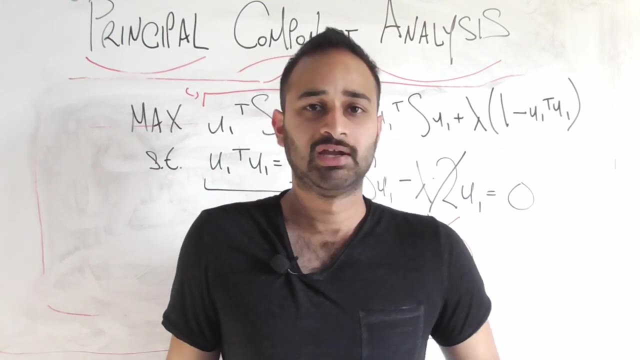 That's a lot. That's a lot. I will admit that's a lot to process. So if you need to go back and watch this video a couple of times or watch the prerequisite videos a couple of times, I'll also link a couple of external resources. if you learn better in a different way.